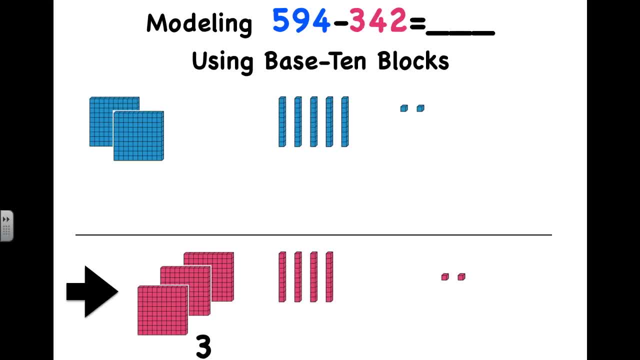 base ten blocks. we have three hundreds, four tens and two ones. So we have taken away the correct amount. We've taken away 342.. So the amount that's left over, the amount that's left over should be the difference between 594 and 342.. So let's see what we. 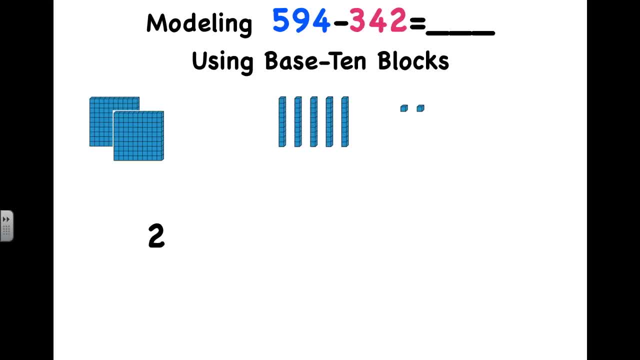 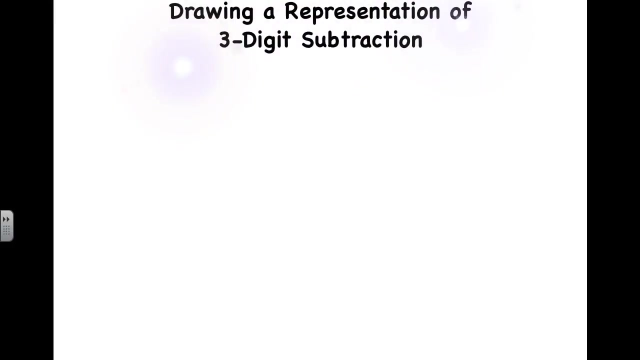 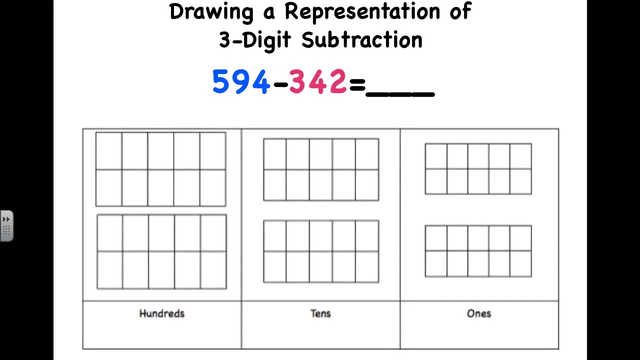 have left over. We have two hundreds five tens and two ones. So this means the difference between 594 and 342 is 252.. Next let's look at how to draw a representation of the same three-digit subtraction problem. Again, we're looking at 594. take away 342.. So we've already represented the problem using 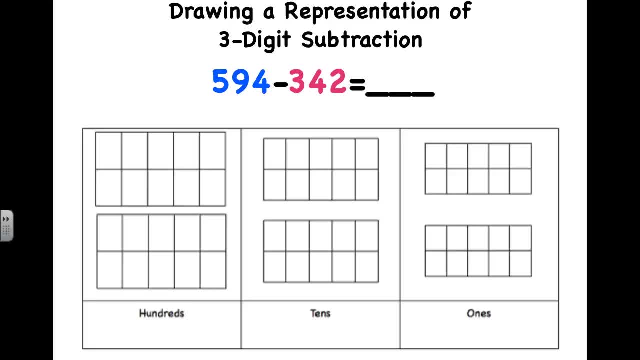 base ten blocks. Now let's look at how this is drawn using paper and pencil. So we'll build 594, just like we did with the base ten blocks, except we'll draw it. So we have five hundreds one, two, three, four, five hundreds, nine tens and four ones. Now we're. 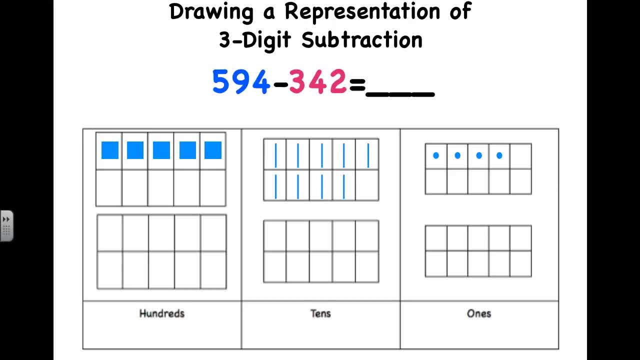 taking away 342.. If you remember correctly, what place do we start taking away from first? If you said the ones, you're correct. So 342 says we take away two. What place do we start with these ones? One, two. So we're just going to mark a neat slash line through the 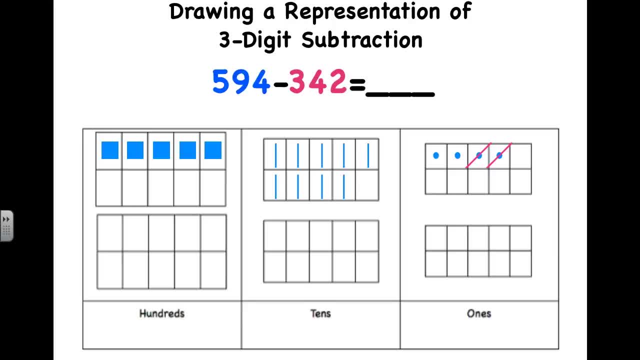 ones that we're marking out. So we've taken away two ones. Next, we need to take away four tens, So one, two, three, four And lastly we need to take away three hundreds. So if the ones- tens and hundreds, going the opposite way on our ten frame. 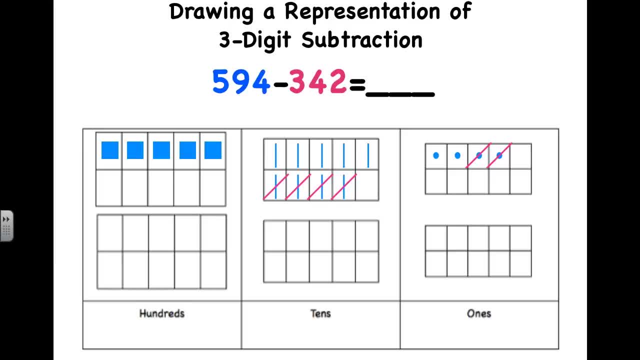 So from bottom right to left and you mark out the numbers until you mark out that entire row, and then you go from top right to top left. So it's the opposite way that you would read a book or complete your rocket math problems.